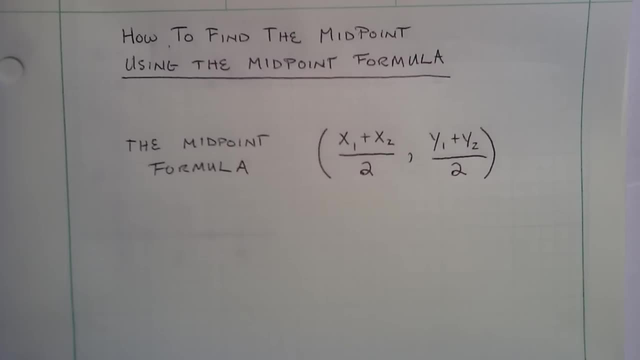 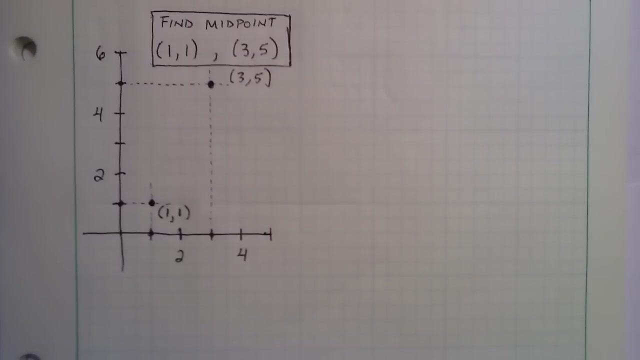 But the midpoint formula is used when we want to find the center of a line segment or the point that is directly in the middle of two other points. So let's go ahead and start our example here. We're going to find the midpoint between the points 1, 1 and 3, 5.. 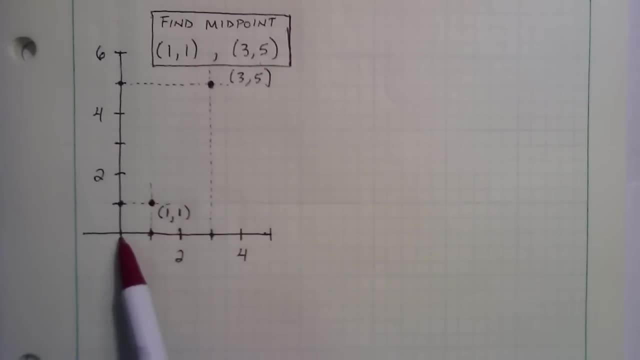 I already went ahead and plotted both of these points. As you can see, this has an x component of 1, a y component of 1, so where those two projections cross is the point 1, 1.. This one has an x component of 3, so you go over 1,, 2, 3 on the x-axis. 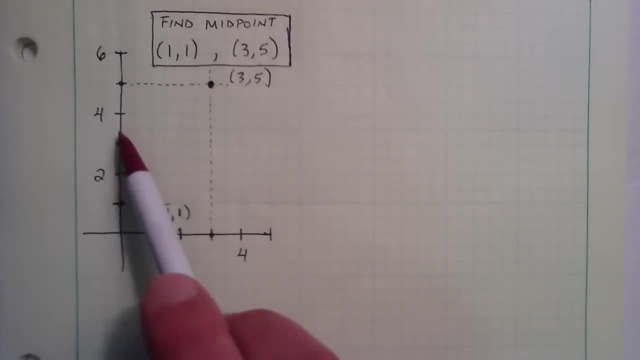 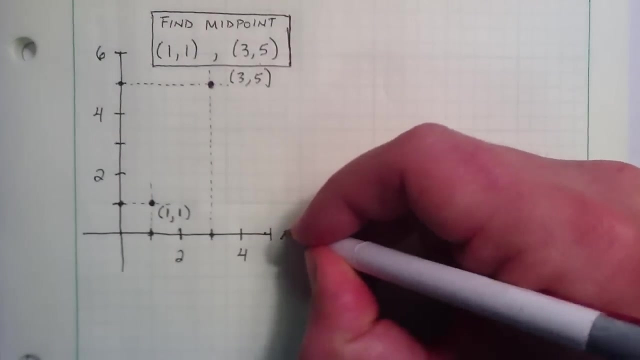 and you go up 5 on the y-axis- 1,, 2,, 3,, 4,, 5, and where these two projections cross, gives you the point 3, 5.. And let me just go ahead and label this x and y, so it's clear. 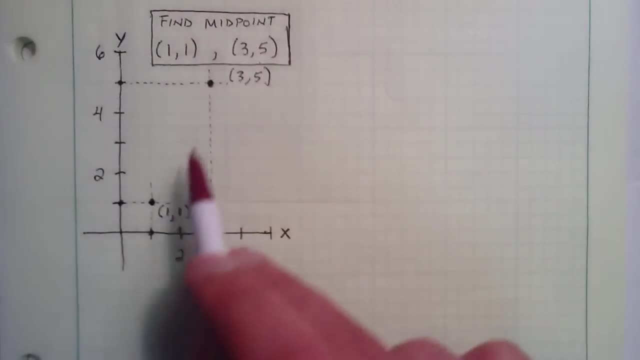 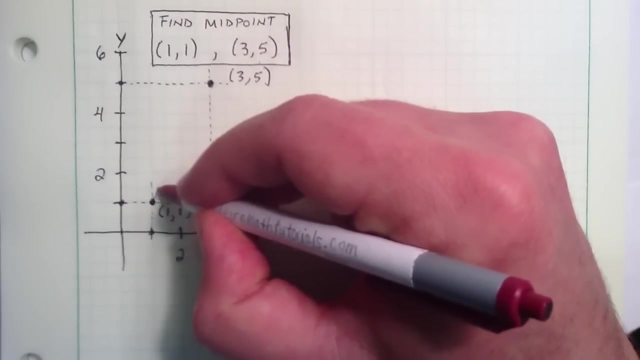 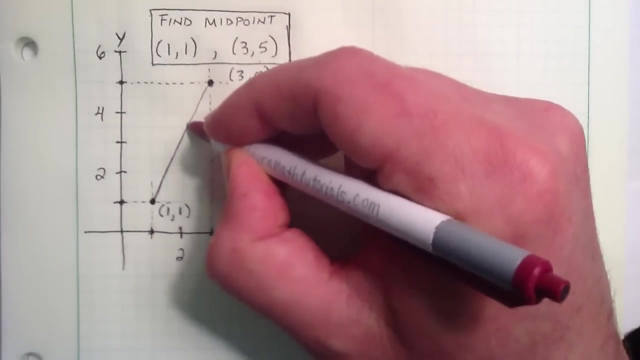 So we want to find the midpoint between these two points, And the answer is actually going to be the same as the center of the line segment connecting these two points. So, either way you want to think about it, The point that's directly in the middle of these two or the center of this line segment. 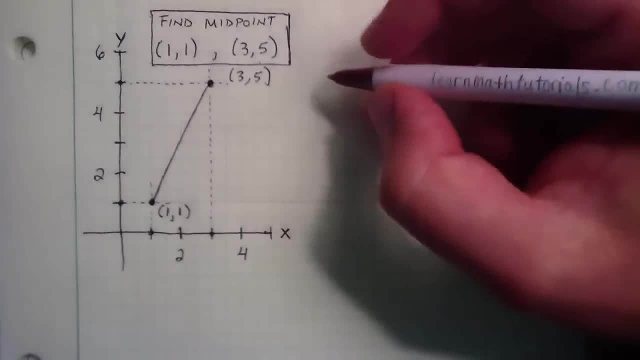 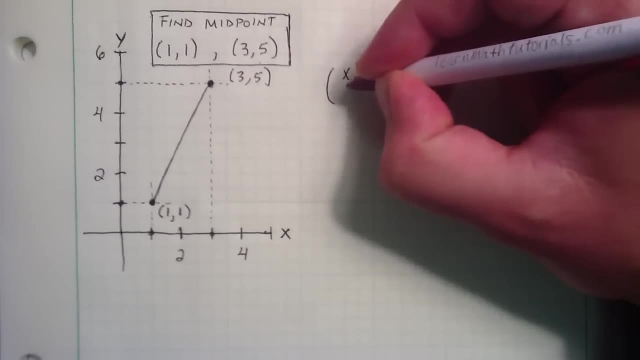 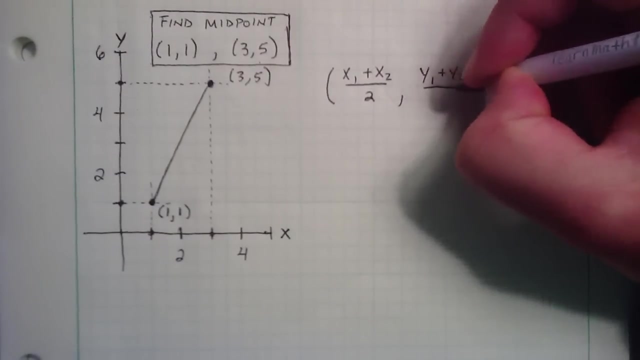 So either one you're looking for, it'll give you the same answer. So let's go back to the midpoint formula. It was x1 plus x2 divided by 2, comma: y1 plus y2 divided by 2.. So really, this is in the form of a point. 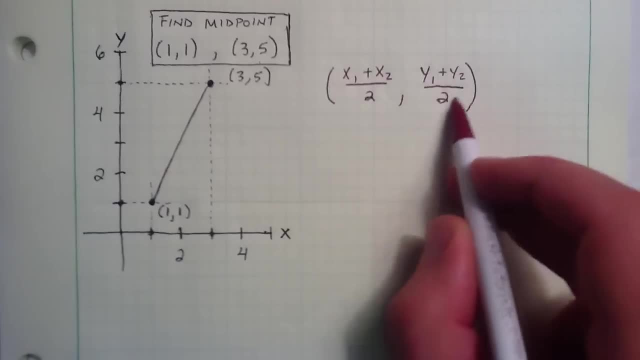 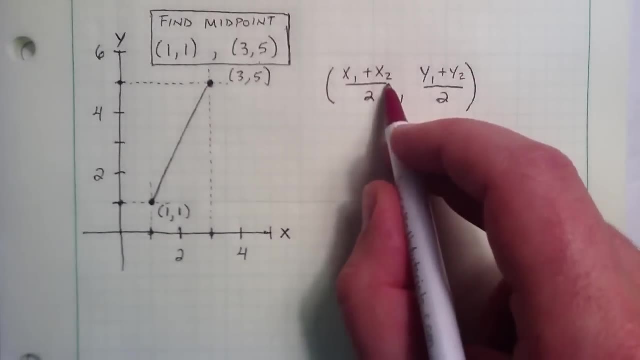 This is the x component, This is the y component of the point And this is the y component of the midpoint. So basically, we just need to figure out what our x1,, x2,, y1, and y2 are, and then we can simplify. 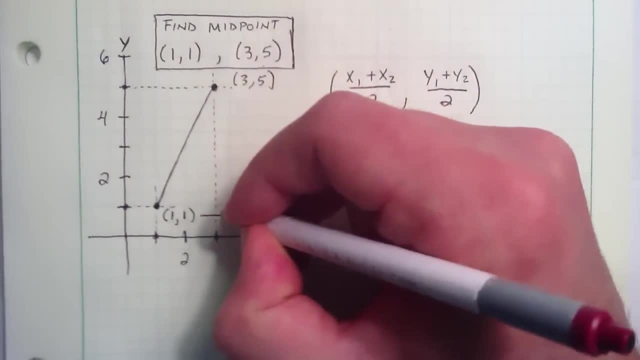 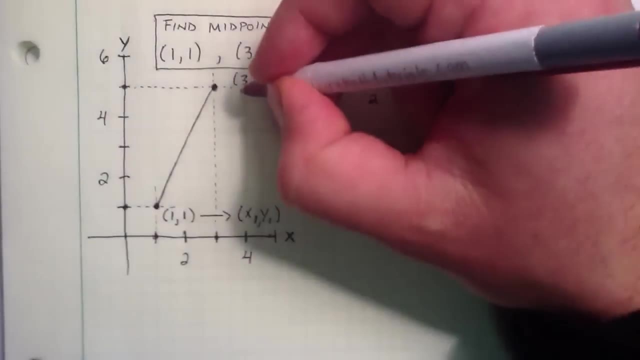 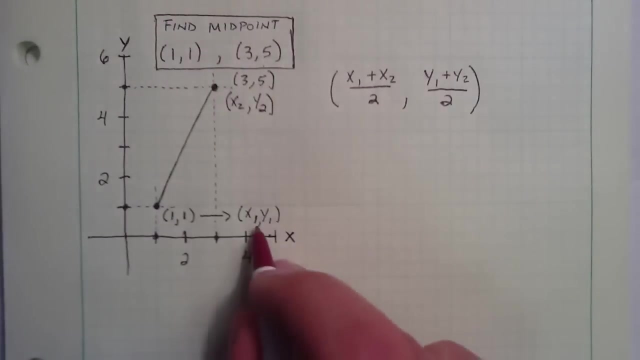 So we're just going to go ahead and rename this point x1, y1. And this one we're going to rename x2, y2.. So I could have named. I could have named these ones x2, y2.. And these ones x1, y1. 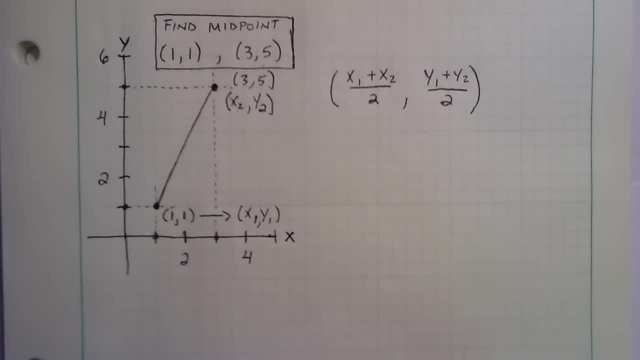 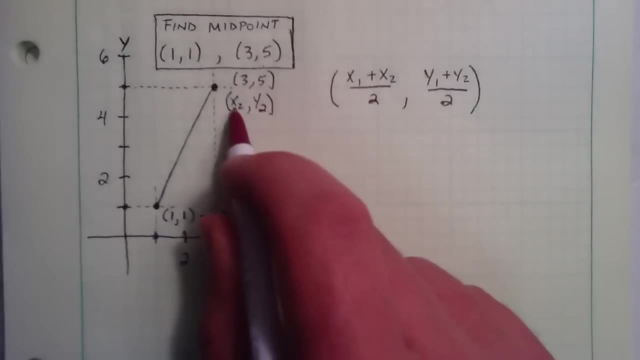 And it doesn't really matter which way I do it, And the midpoint formula is going to give you the same answer either way. So just take your pick. As long as one of them is both 1s and the other one is both 2s, you'll do fine. 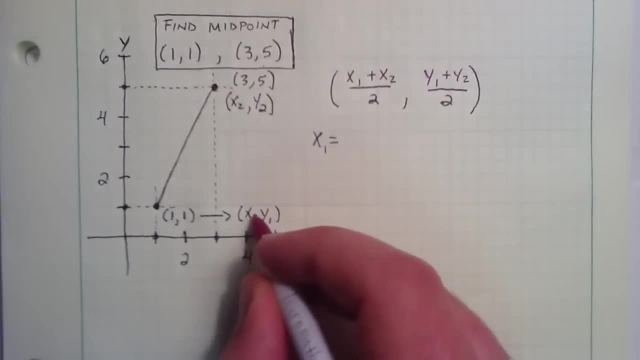 So let's go ahead and write down x1 here Now. x1 is the left-hand side or the x component, So it refers to the left-hand side or the x component. So it refers to the left-hand side or the x component. 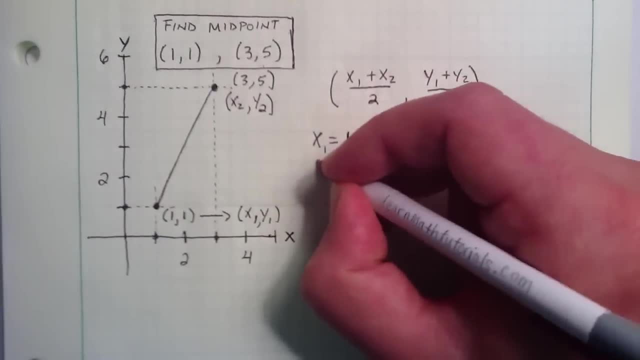 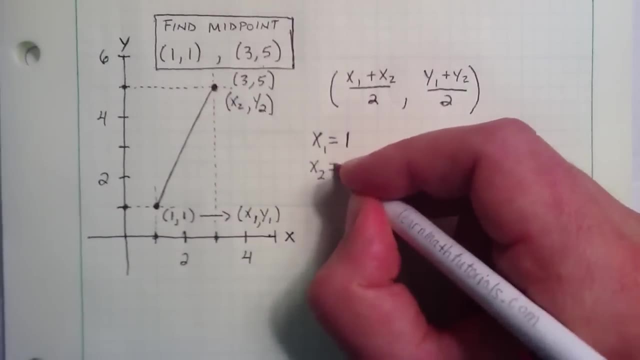 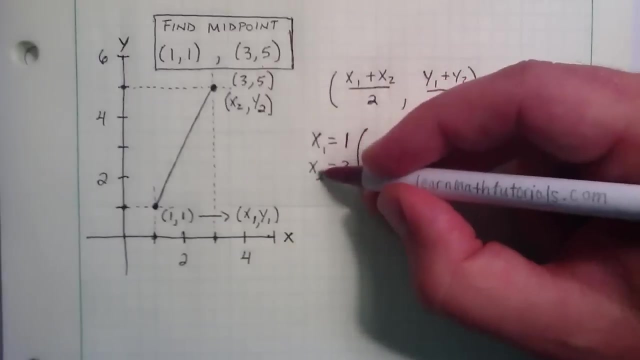 component of this point, which is a 1 and X 2, refers to the X component or the left-hand side of this point. so that gives us the 3. so now we can build the X component of our midpoint. X 1 plus X 2 is simply just 1 plus 3, and then that's. 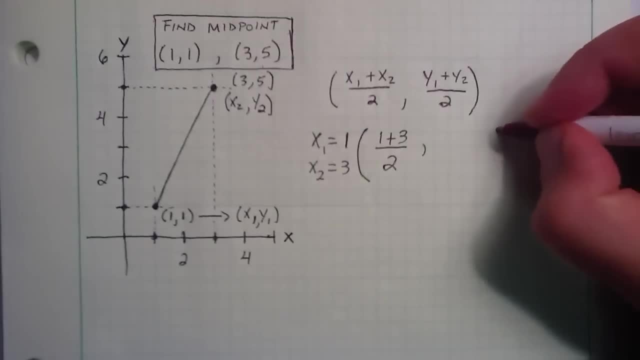 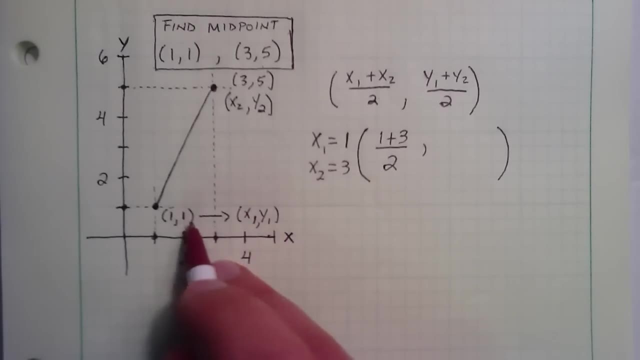 divided by the 2, and so now we want to find our Y 1 in our Y 2, and so Y 1 refers to the right-hand side or the Y component of this point, which is a 1, and the Y 2 refers to the right-hand side or the Y component of this point. so that's. 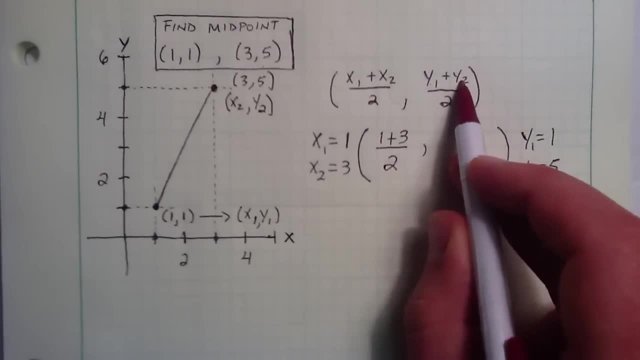 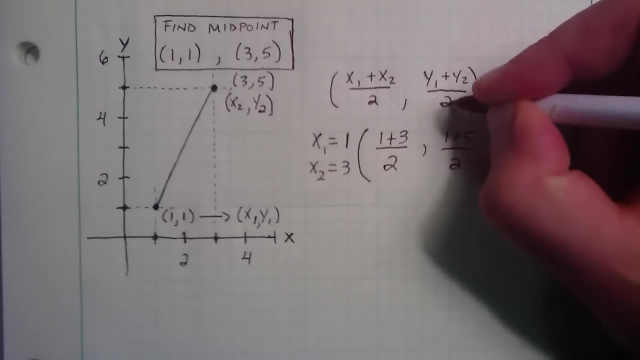 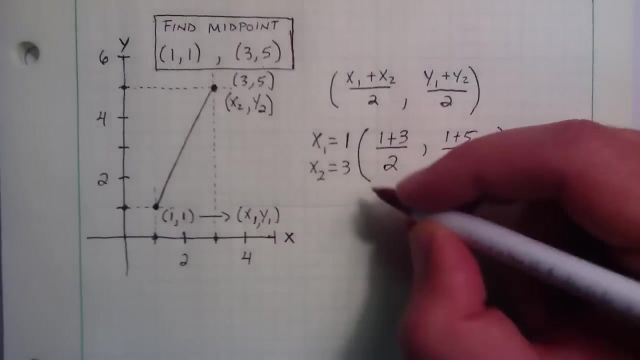 a 5. so then really, Y 1 plus Y 2 is simply 1 plus 5, and then that's divided by our 2.. So we have the midpoint, but let's go ahead and simplify it: 1 plus 3 is simply 4, and then that's still divided by the 2.. 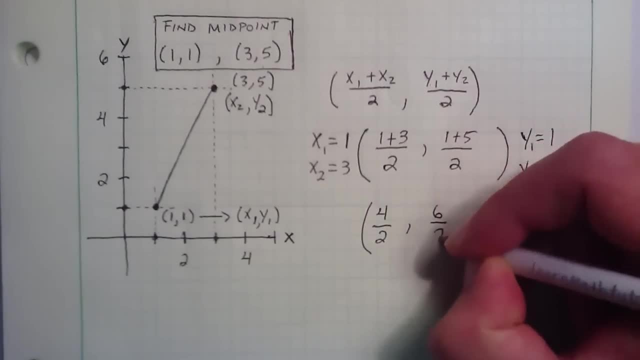 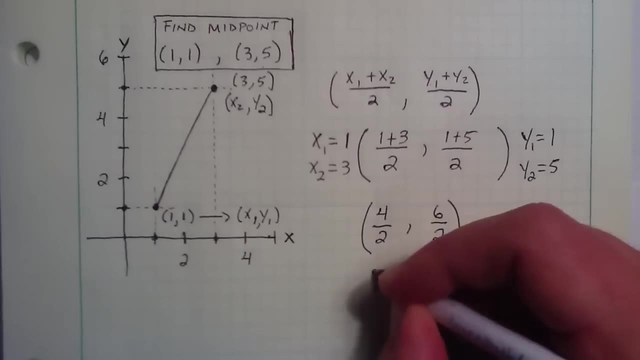 And the 1 plus 5 is a 6, which is divided by the 2.. And we can further simplify: 4 divided by 2 simply gives us 2.. 6 divided by 2 gives us 3.. And there we have it. 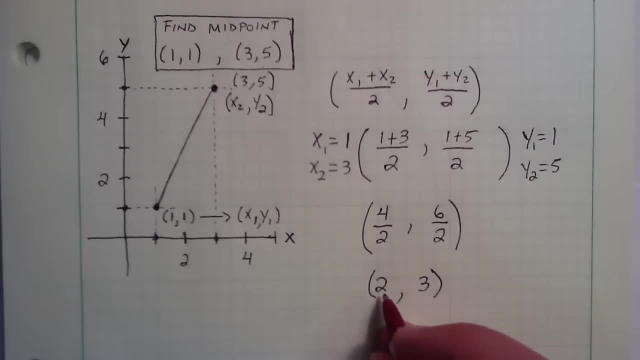 We have our simplified midpoint, And so this is going to be the point directly between these two points, or in the center of this line segment. So let's go ahead and plot it. This has an x component of 2.. So, starting on the x-axis at 0,, go over 1,, 2..